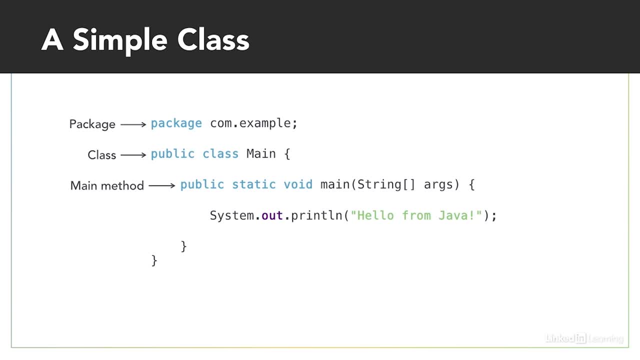 of the main class in order to run this method. Void, which means that the class doesn't return anything, and then the name of the method. Within the parentheses, you define parameters. These parameters are designed to receive data as the method is called. The main method is defined strictly in command-line applications. 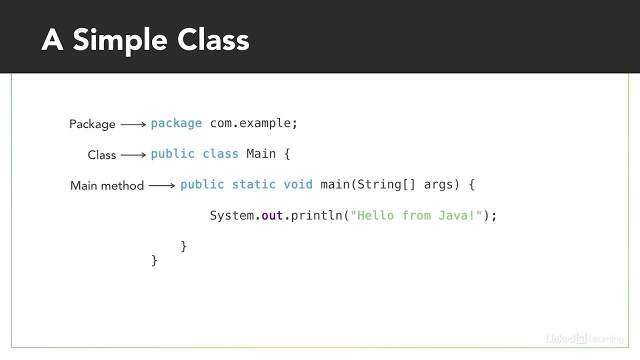 as the method that's executed automatically when you start up the class, And it always receives an array of string values. Finally, you have your executable code. This main method only has one line of code, but you can actually have as many as you want. 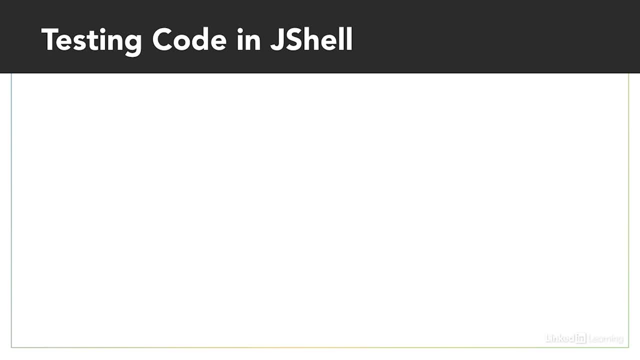 So this is a simple but well-formed class that will run successfully on the Java Virtual Machine. You can also test your Java code in JShell, a command you can run from terminal on Mac or from a command window on other operating systems. JShell was introduced with Java 9,. 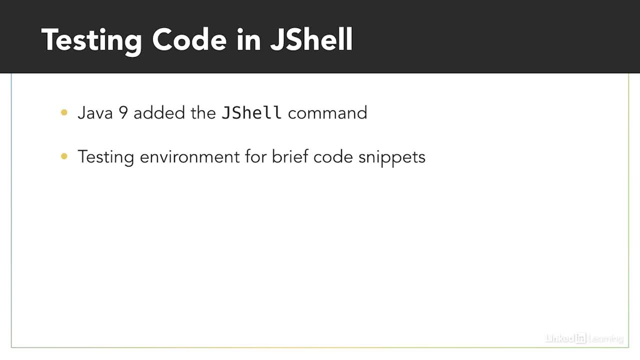 And it lets you just test your code before you take that code and put it into a fully formed class In JShell. you don't need a complete class. You can just execute one line of code at a time And then you can take that code that you've tested and 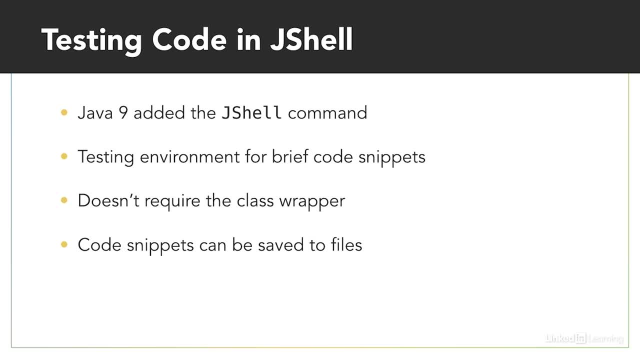 save it out to a file so you can convert it to production code. In Java, everything is case sensitive, So your identifiers, such as variable, method and class names, all need to be unique within their particular scopes Because of this case sensitivity. 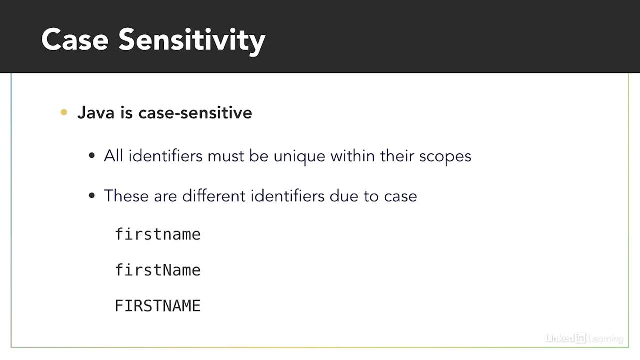 the following are different identifiers from the Java point of view. They all say first name, but the first one is lowercase, the second one uses camel case and the third is all uppercase. These are each seen as unique. Java in general is not sensitive to white space. 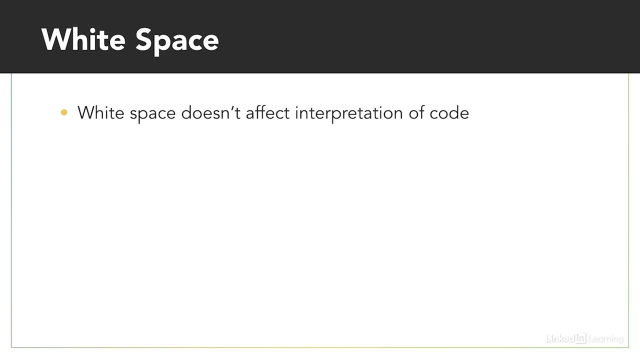 That is to say, extra white space doesn't affect how your code is interpreted or compiled. And in fact if you put in extra spaces, tabs or line feeds, those will be collapsed by the compiler. Let's say you have five line feeds. 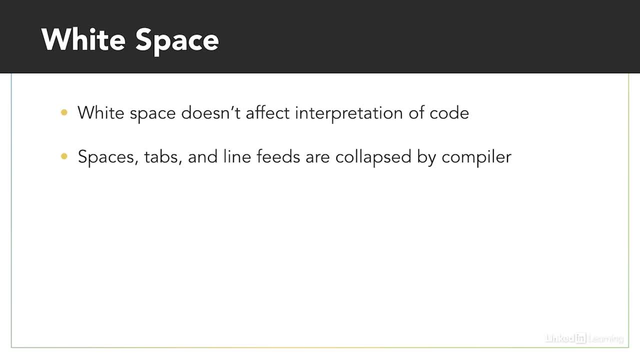 From a compilation point of view, that's the same as one line feed. In order for this to work, all statements in Java must end with a semicolon character. So, for example, this is a bit of code that outputs a string. hello from Java to the console. 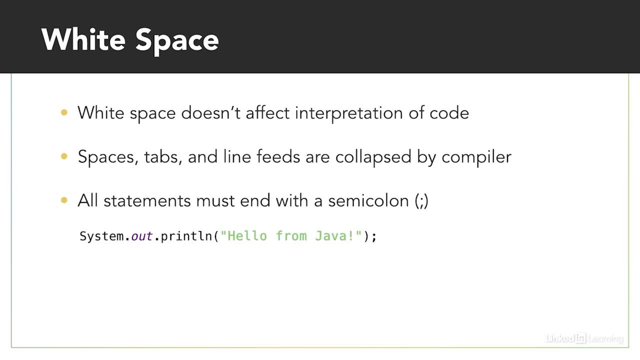 And because it's a single statement, it ends with that semicolon character. If you're working on a full-blown class and you forget the semicolon, it'll cause a compilation error. If you run this same command, though, in JShell, it'll work fine without. 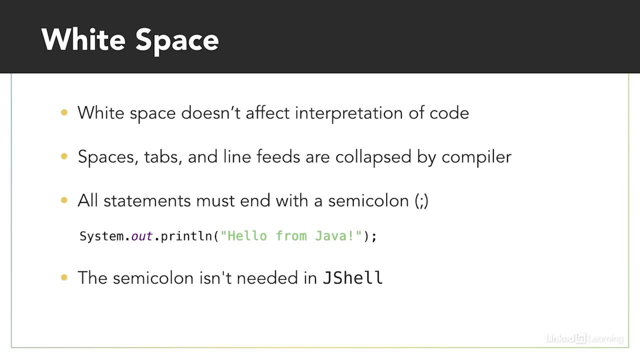 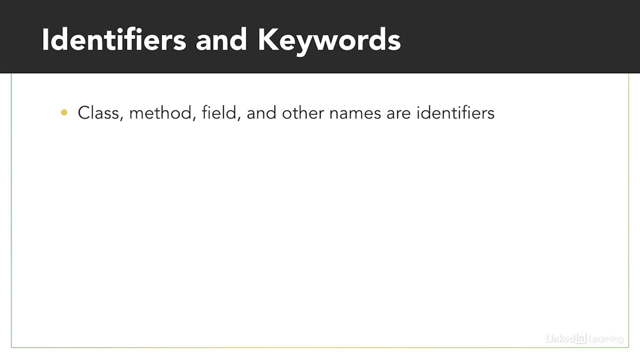 the semicolon, because semicolons aren't really needed in JShell Or, to put it more accurately, they're added automatically for you in the background. There are some very strong conventions that are used by all Java developers, and you should follow these conventions. 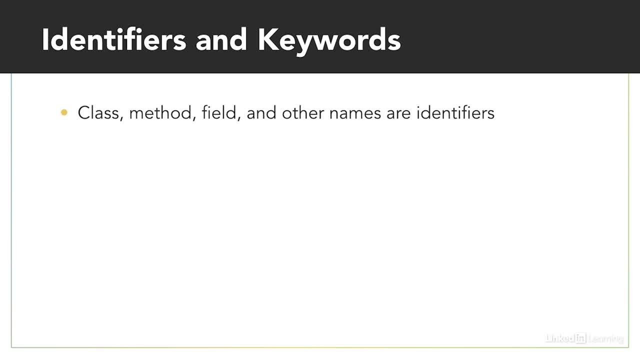 First of all, there's an absolute, absolute requirement that all identifiers must start with either an alphabetical character A through Z or an underscore character. You can't use numbers as the first character in an identifier. You also can't use keywords as identifiers. 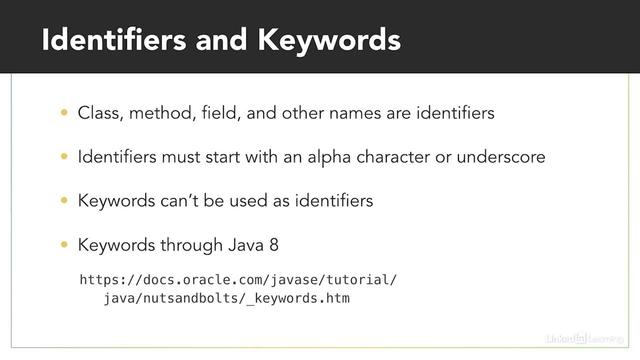 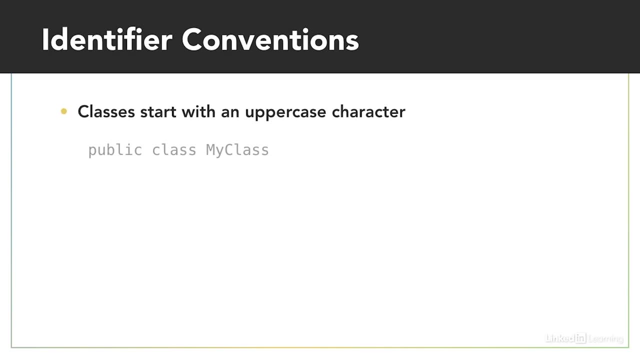 You can find a comprehensive list of Java keywords up through Java 8 at this webpage, and then you can look at the documentation for more recent versions of Java to find out what keywords have been added since then. There are some very strong conventions for creating your identifiers. 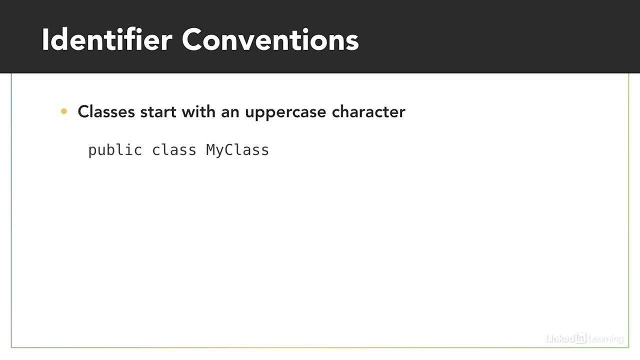 Class names always start with an uppercase character, but then use mixed case for the rest of the class name. Methods and variables always have names that start with a lowercase character. So when you look at an identifier, you can distinguish between a class name and. 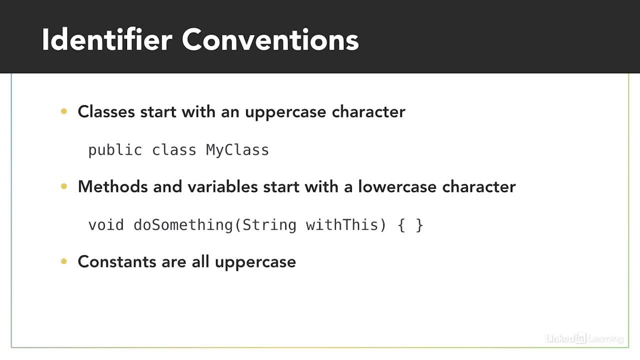 say a method name or a variable name. Constants are an interesting situation with Java. There isn't really any such thing as a pure constant. in Java. There are these two things. One is there isn't a keyword such as const. Instead, in order to define a value that never changes, 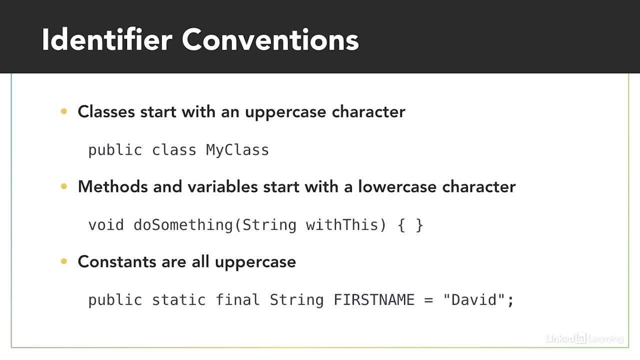 you start with the keywords public, static and final, And then the data type- string in this case- and then the identifier- Constant identifiers are always spelled in all uppercase. Now, all of these are just conventions. You could do it differently if you wanted to, but it's a great idea to follow. 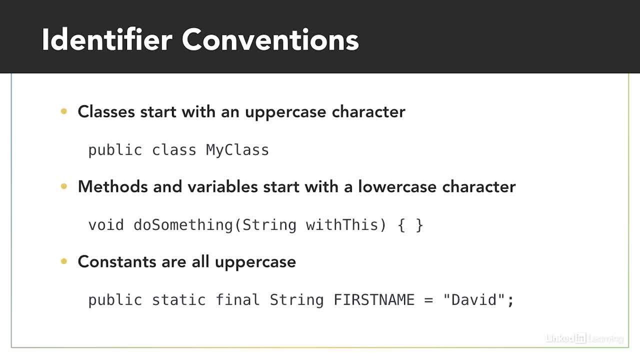 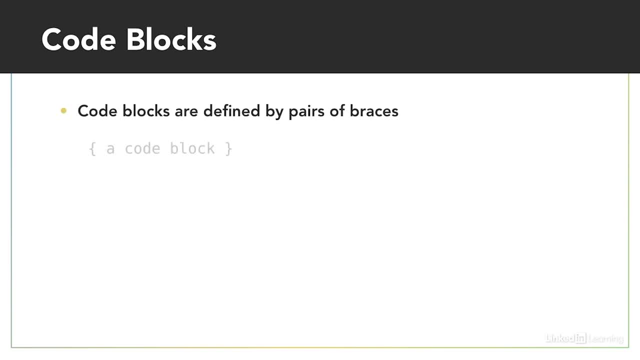 the conventions that have been established and are followed broadly within the Java development community. Finally, I mentioned code blocks. A code block is defined by a pair of braces. This is a way of organizing your code, but it's also a way of restricting visibility of variables.